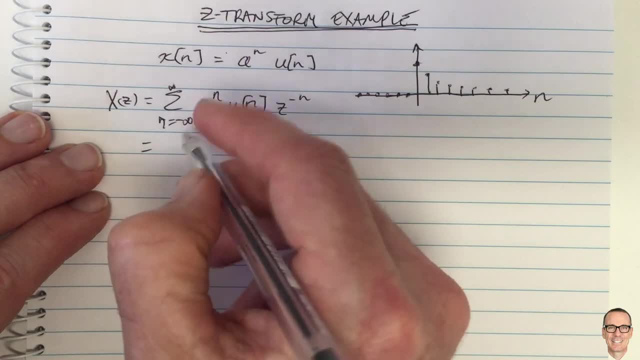 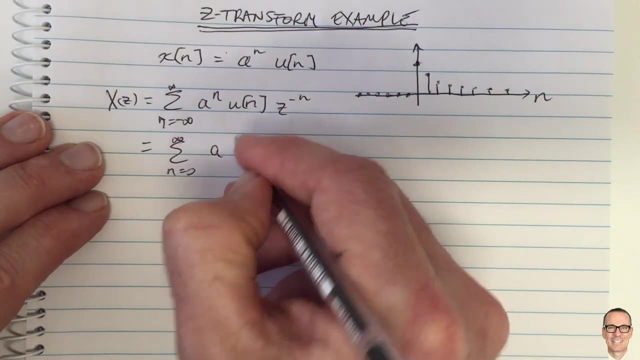 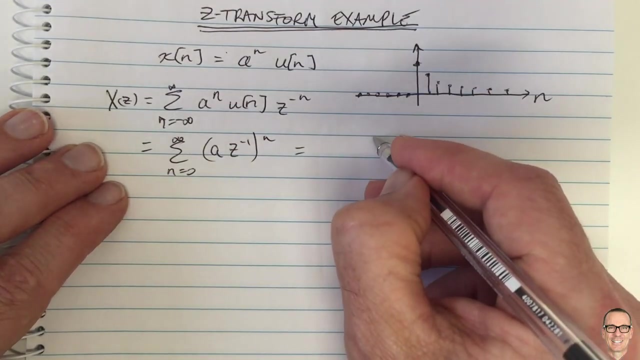 This is the formula for the Z-transform, And so this equals, because of the un function, we can sum from 0 to infinity, Of a z to the minus 1 to the power of n, And this equals- it's an expression that can be looked up- that that summation is a times z to the minus 1.. 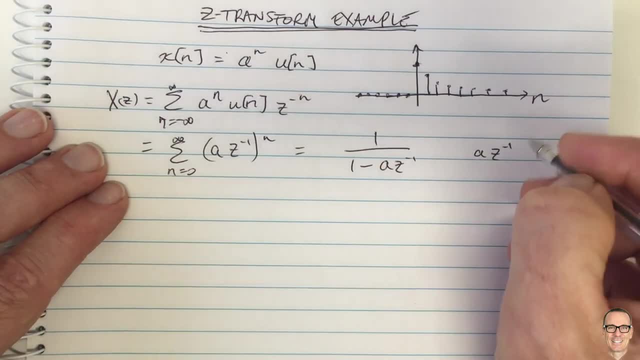 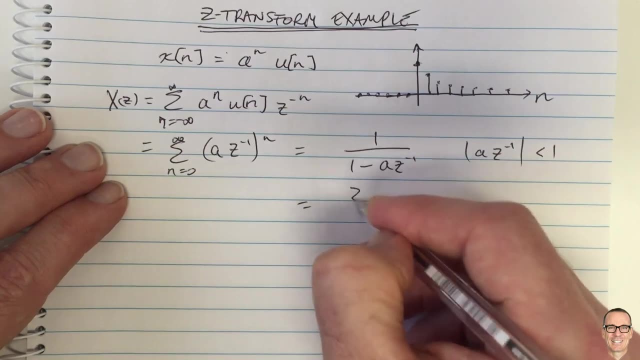 Where, for as long as a z to the minus 1, as long as the mod is less than 1.. OK, so this also, we can multiply top and bottom by z, So we have z on z minus a And we rearrange this. 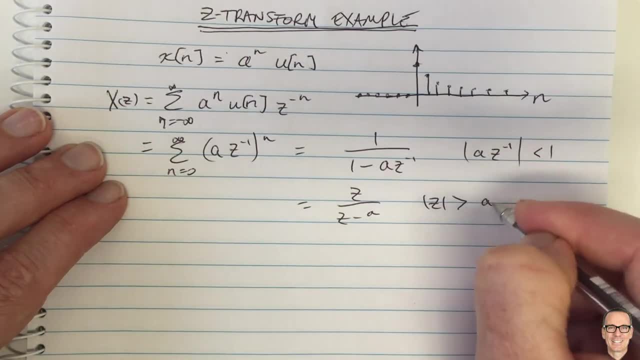 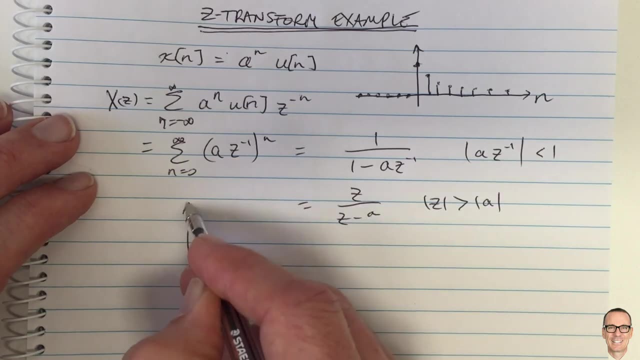 We can see that the mod of z has to be bigger than the mod of a. So this is the answer. And then we also just consider what's happening in the z-plane. What does this? where does it converge? Where does this hold? 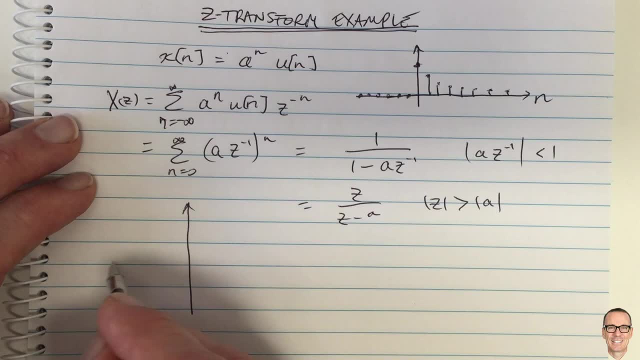 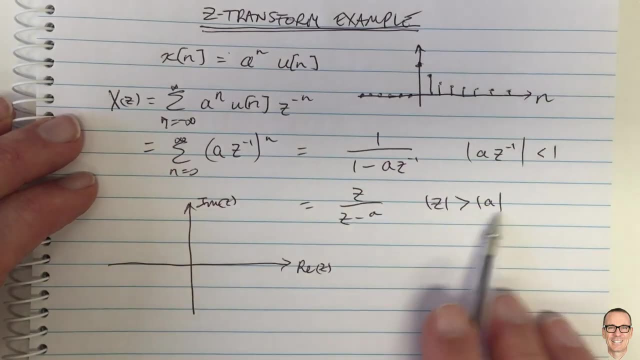 This summation converges as long as this holds. So, in the z-plane, we have the real part of z, the imaginary part of z And this mod, The mod of z being less than the mod of a, it defines a circle. 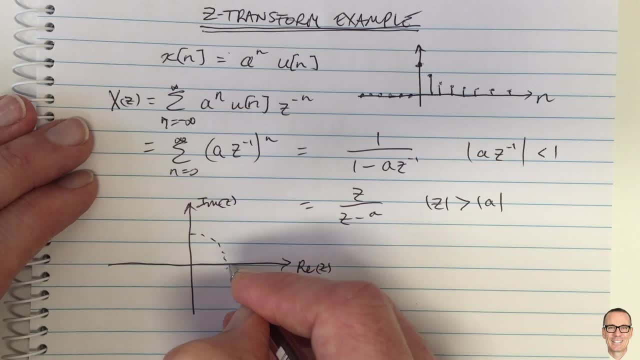 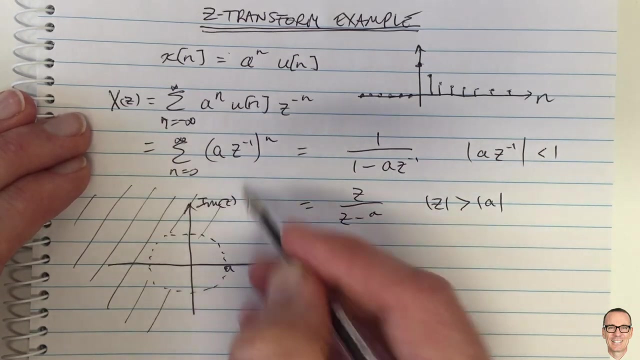 So there's a circle here of radius a, Where, if we are outside that circle- because mod of z has to be bigger than mod of a, If we're outside that circle, then we know that this function, this summation, this infinite summation converges. 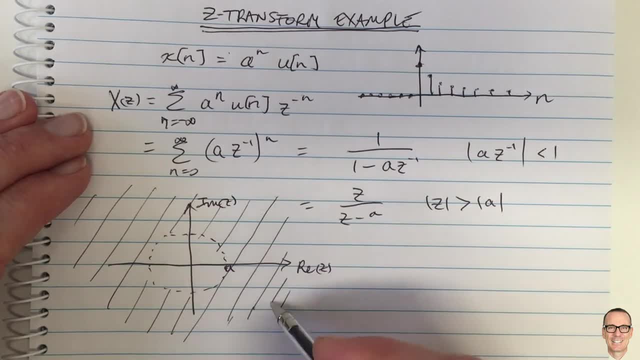 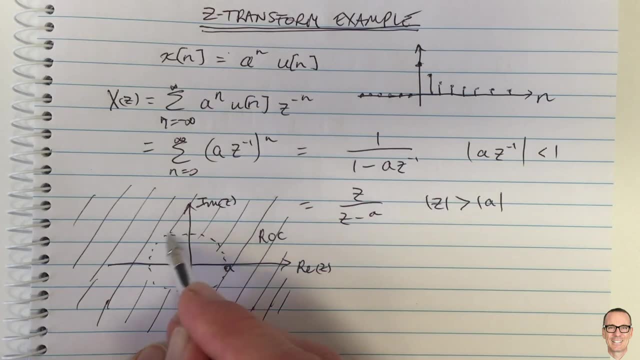 And therefore our z-transform holds. So our z-transform Holds in this whole region of convergence And for z-transforms it's a circular boundary on the region of convergence And there's a pole at z equals a, Because if z equals a, you get an infinite value here. 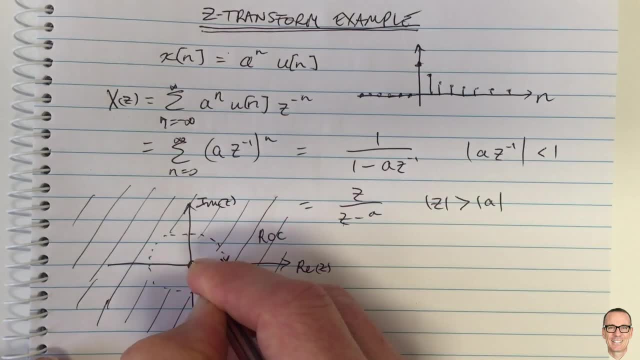 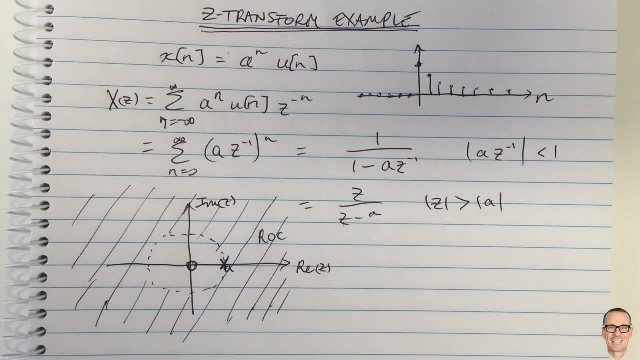 And there's a zero at z equals zero In the z-plane, So don't forget to like this video And subscribe to the channel For more videos on signals and systems.